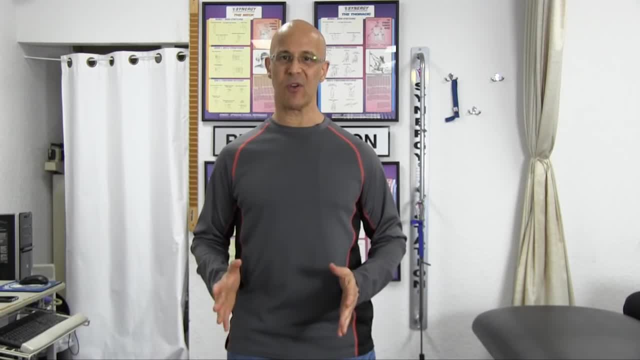 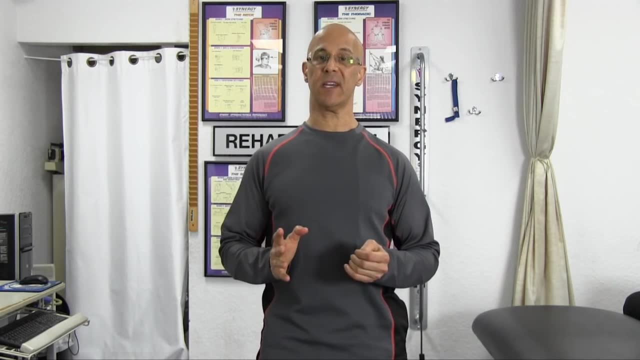 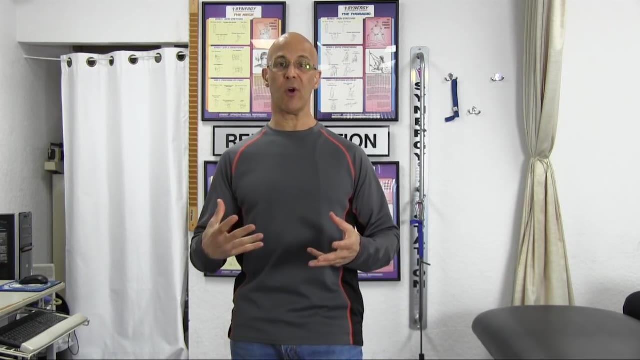 who stand more are those that are more slimmer than those who sit more. The concept non-exercise activity thermogenesis: a study in 2005, Mayo Clinic. they state that people that were standing two hours more per day than sitting were burning more calories, and those were the people that 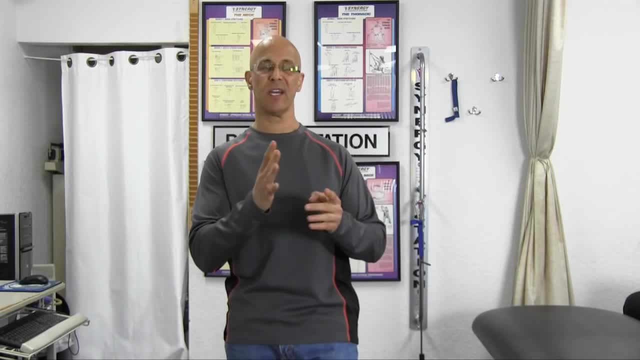 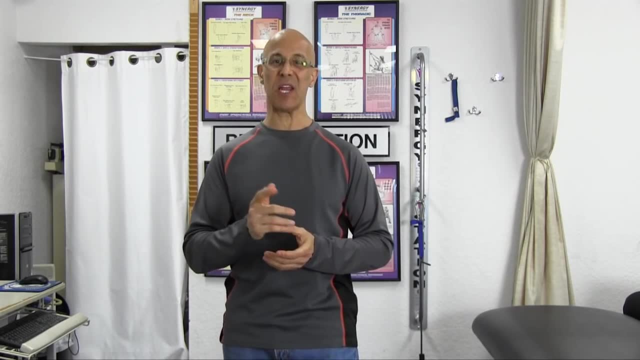 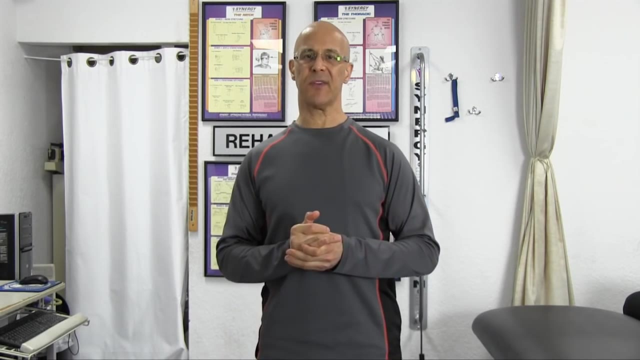 had less fat. Now this actually went back to our ancestors back years ago, that there was no fat people around. although they were not sitting either, They were always standing while eating. An interesting article in the Journal of Endocrinology and Metabolism 2013,. 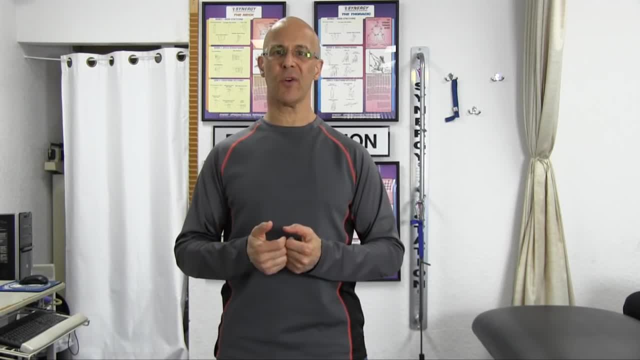 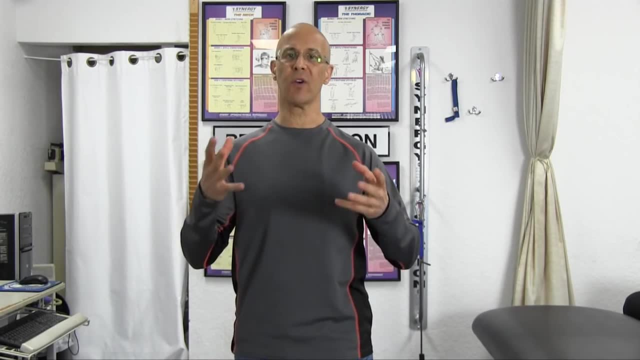 it takes 20 minutes for our brain to know if we're full or not. So, therefore, people who eat fast are those that are never going to know if they're full. So what does that mean? It means that you're over-consuming more food and your brain is not understanding. 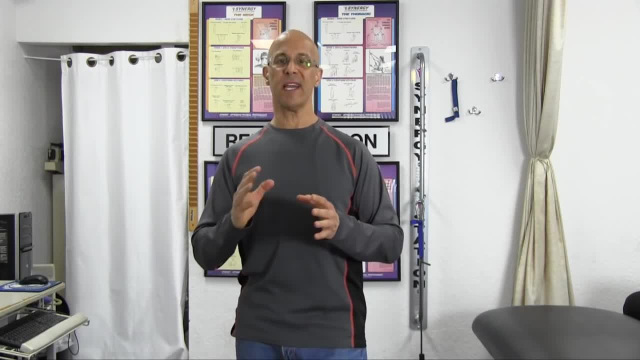 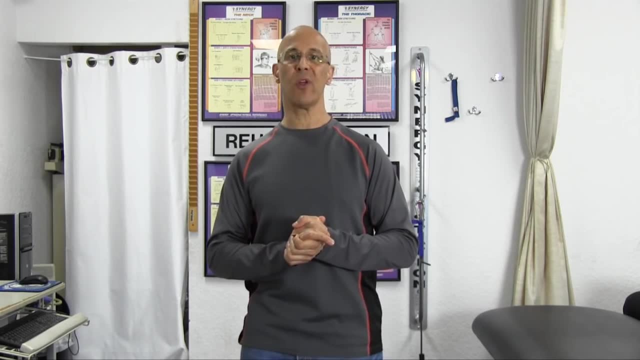 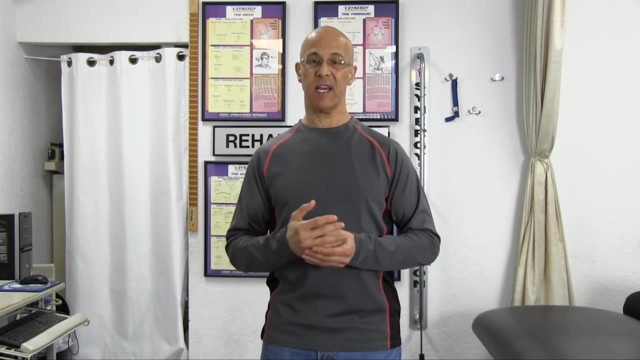 how much food it's in is in your tummy, So eat slower that within 20 minutes, your brain will be able to communicate with your stomach and let you know how full you really are. Now standing in itself has a lot of different positive changes when it comes to metabolism. 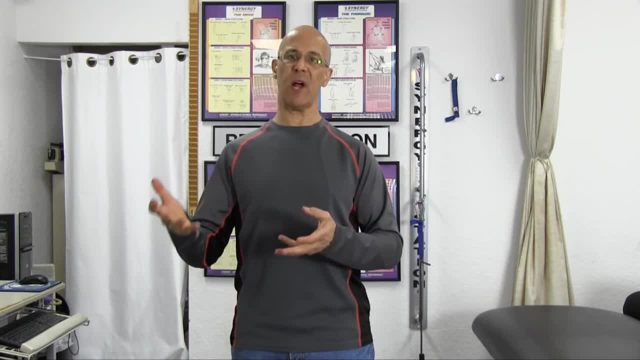 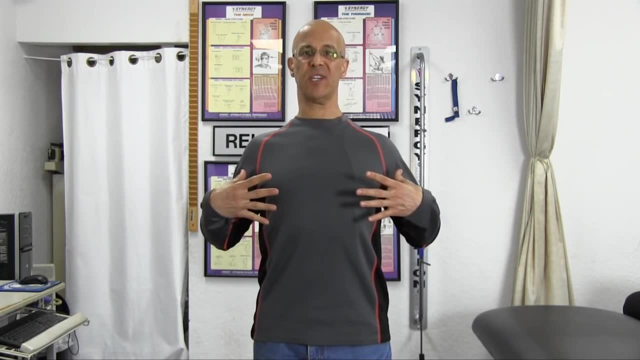 There are different thermogenic factors, certain enzymes that are secreted while standing. as compared to sitting, The bottom line is that you stand. you get more revived, more fresh, more oxygen into the lungs, The joints become more mobile, We have more. 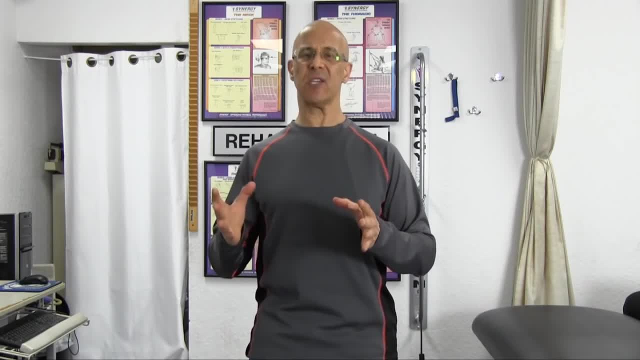 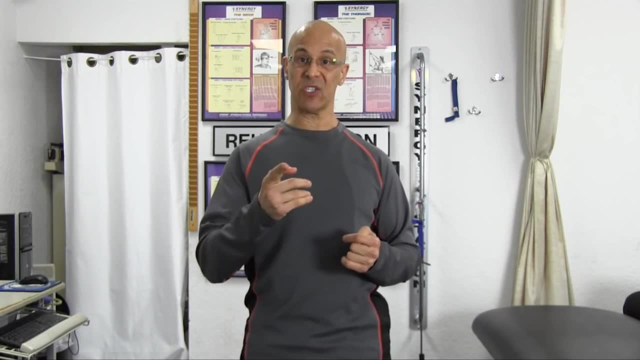 – we have better circulation within our cardiovascular system. Just, things work better. The bottom line is that the people who stand more are people that are going to burn more calories and obviously lose more weight. The bottom line is: you need to get on your feet. When you're standing, you're going. 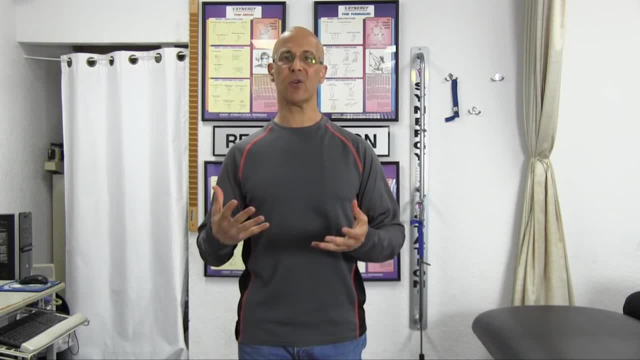 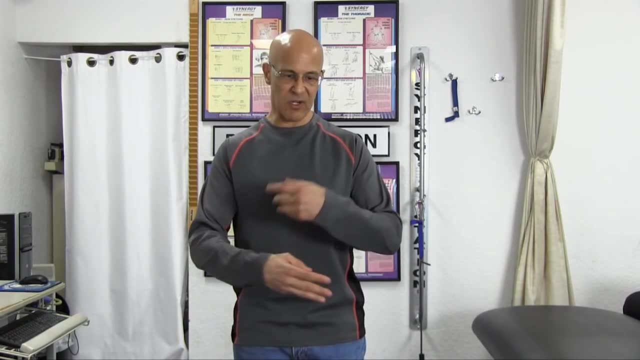 to burn more calories, increase thermogenesis. You're going to increase circulation, have better oxygen. You're going to have better posture. You're going to have better circulation. You're going to have better digestion and everything else You need to get off your. 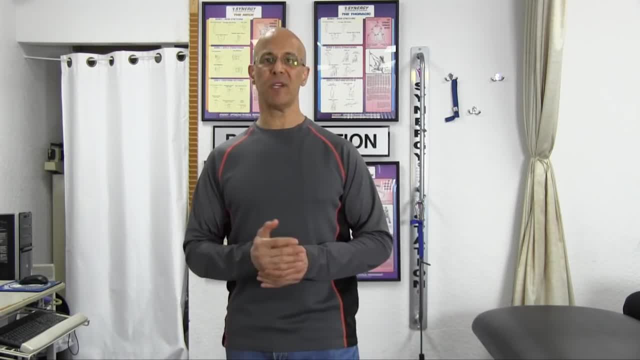 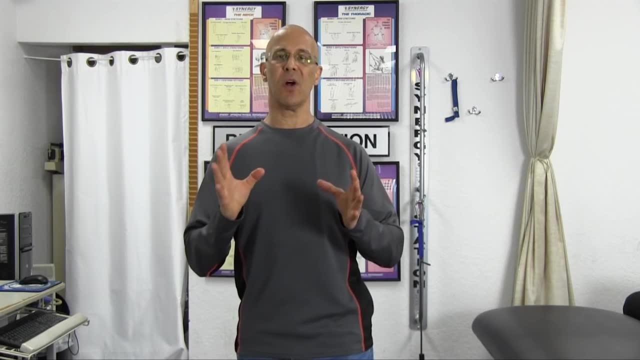 tail And get on your feet. I hope this video has given you a little bit of insight. You may be asking me: well, should I be standing when I eat? Well, I can tell you this: The more you're on your feet, the 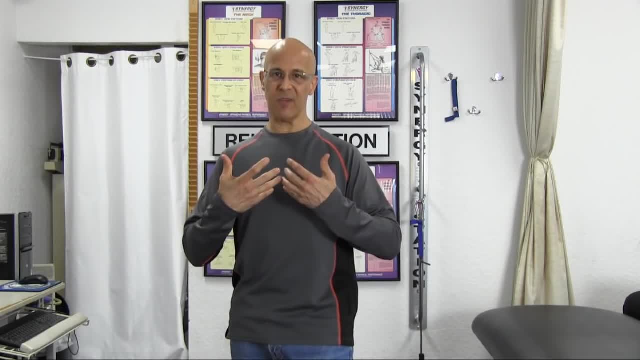 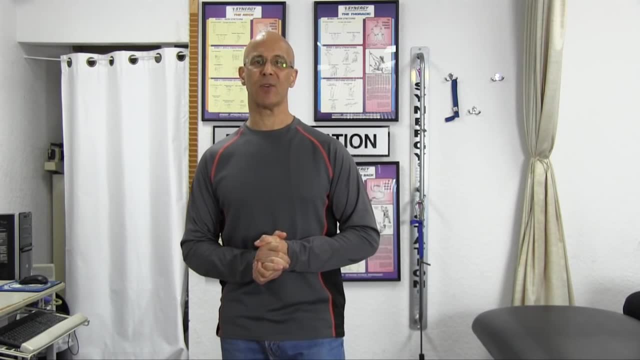 more calories you're going to burn and the more oxygen you're going to get in your system and the more you're going to revive your system as well. So you make that choice. I ask you to make it a great day. I'm Dr Alan Mandel.